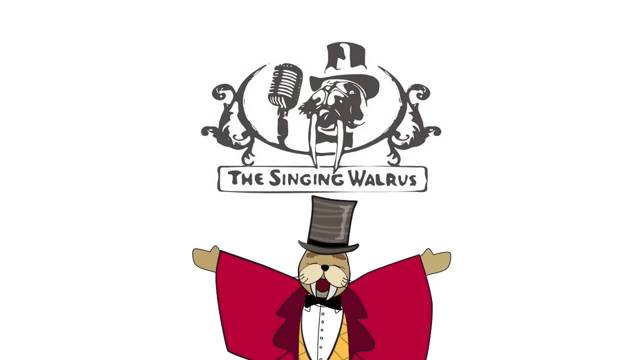 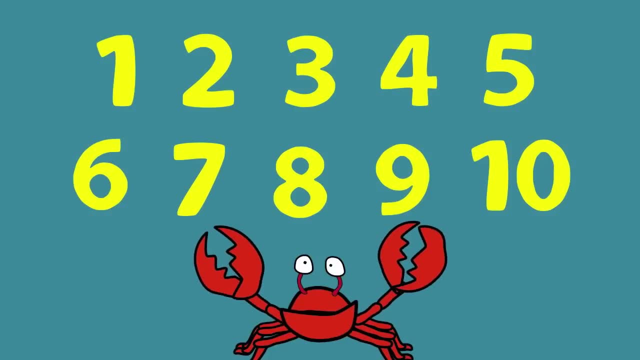 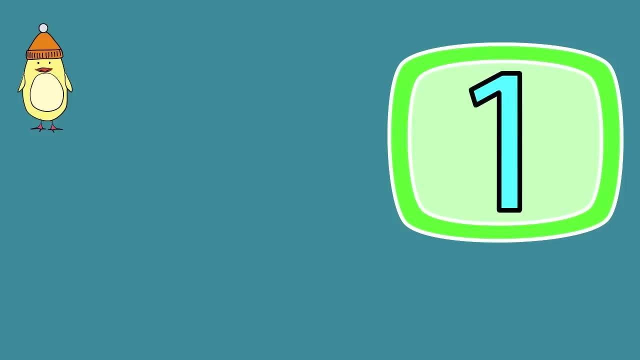 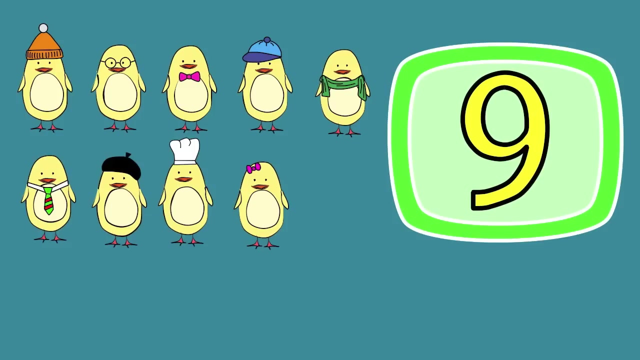 Hi kids, today we're going to learn the numbers 1 to 10.. Do you know how to count from 1 to 10? Let's take a look: 3, 4,, 5, 6, 7,, 8,, 9,, 10.. 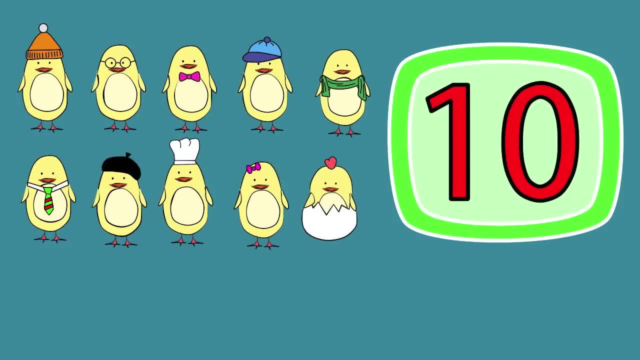 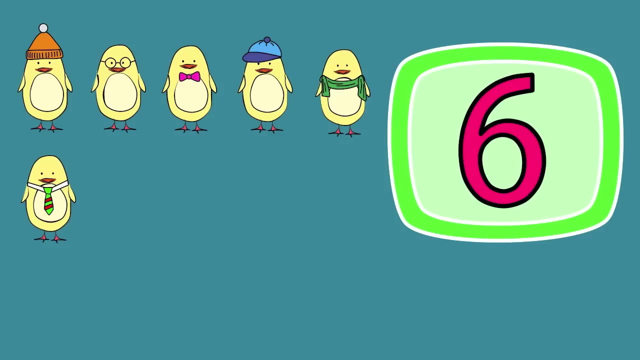 10,, 10.. Okay, now let's count from 10 to 1.. 10,, 10., 9,, 9., 8,, 8. 7,, 7., 6,, 6., 5,, 5.. 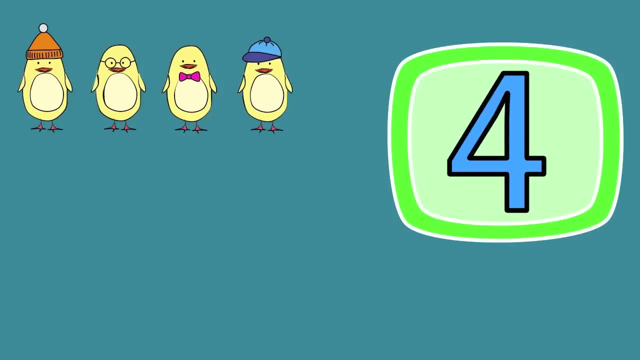 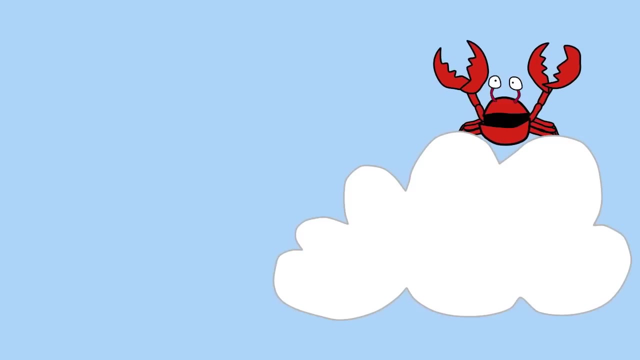 4,, 4. 3,, 3., 2,, 2., 1, 1.. Fantastic, Fantastic. Let's try it one more time: 1. 1., 2,, 2., 3,, 3.. 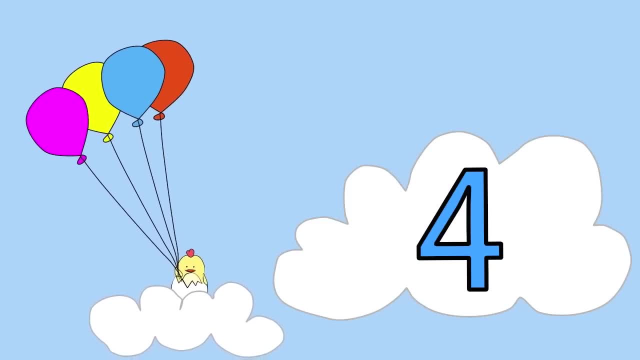 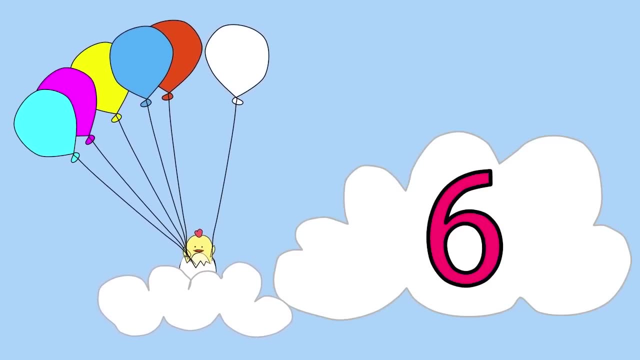 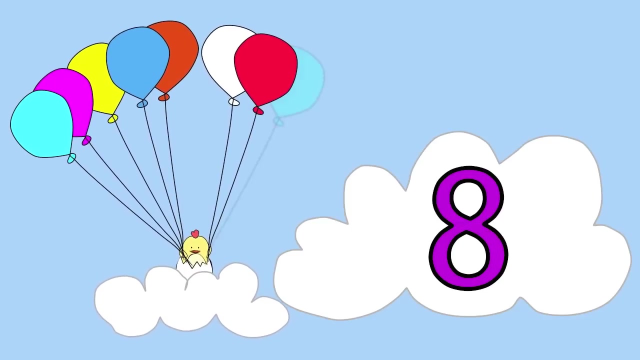 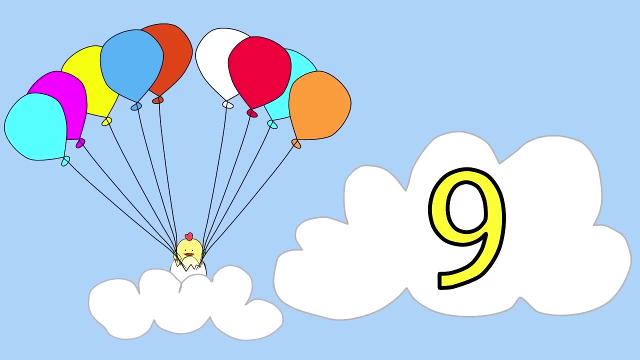 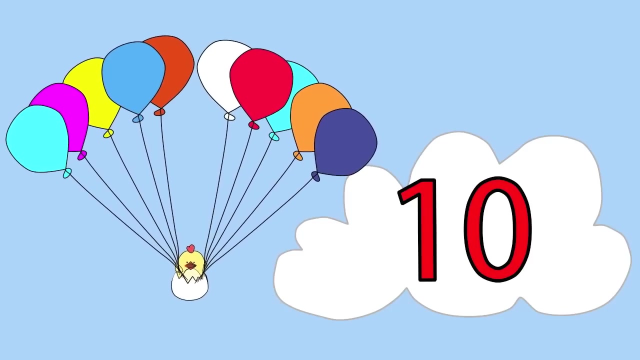 4,, 4., 5,, 5., 6,, 6., 7,, 7., 8,, 8., 9,, 9., 10,, 10. Great, Now let's count from 10 to 1.. 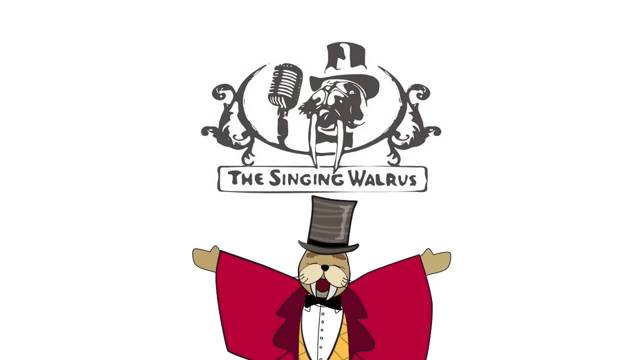 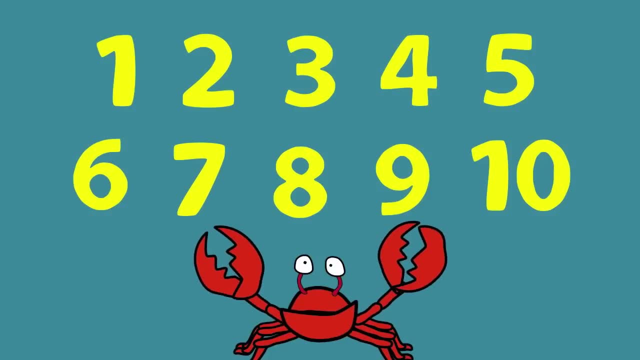 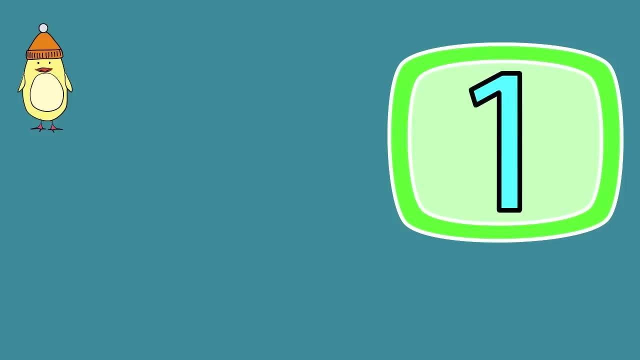 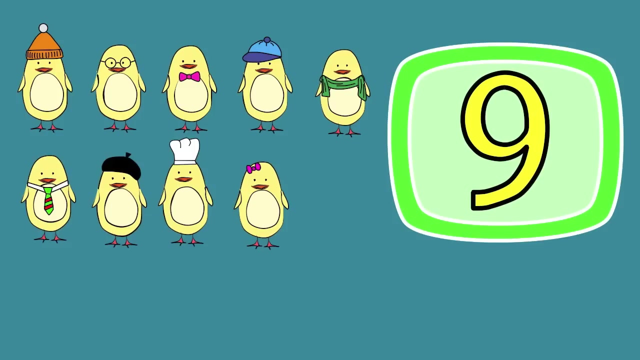 Hi kids, today we're going to learn the numbers 1 to 10.. Do you know how to count from 1 to 10? Let's take a look: 3, 4,, 5, 6, 7,, 8,, 9,, 10.. 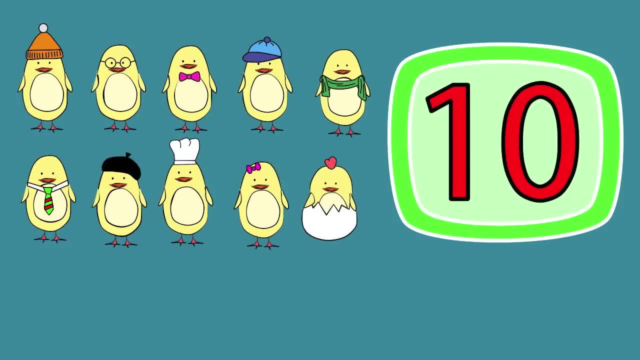 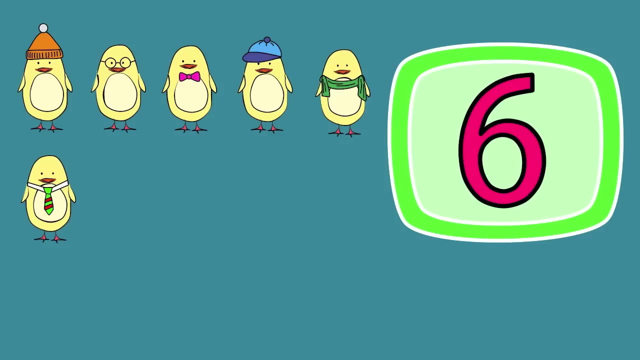 10,, 10.. Okay, now let's count from 10 to 1.. 10,, 10., 9,, 9., 8,, 8. 7,, 7., 6,, 6., 5,, 5.. 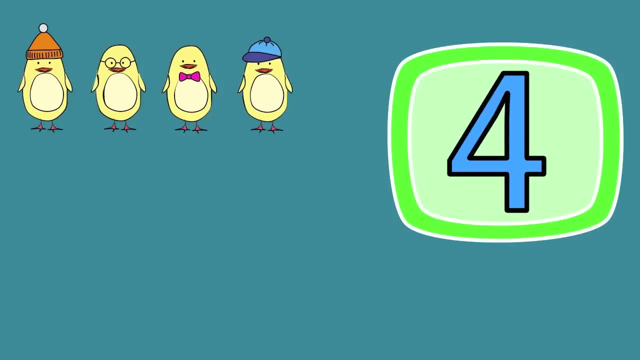 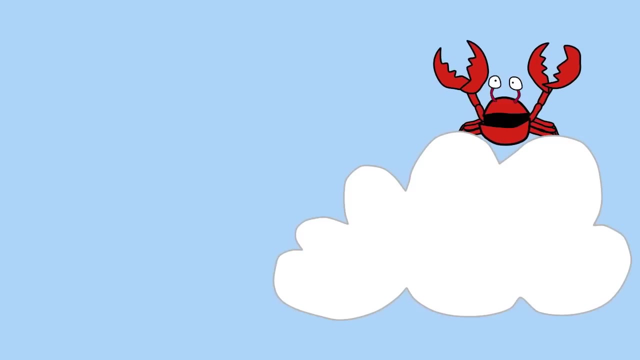 4,, 4. 3,, 3., 2,, 2., 1, 1.. Fantastic, Fantastic. Let's try it one more time: 1. 1., 2,, 2., 3,, 3.. 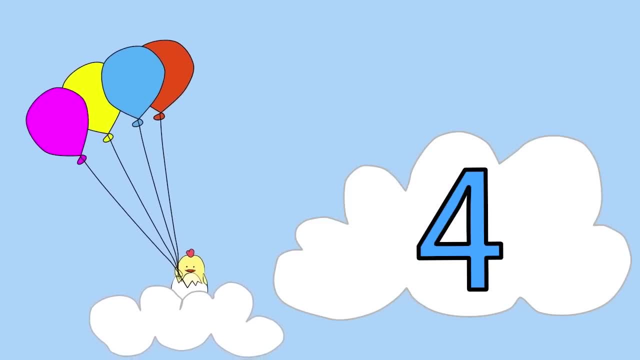 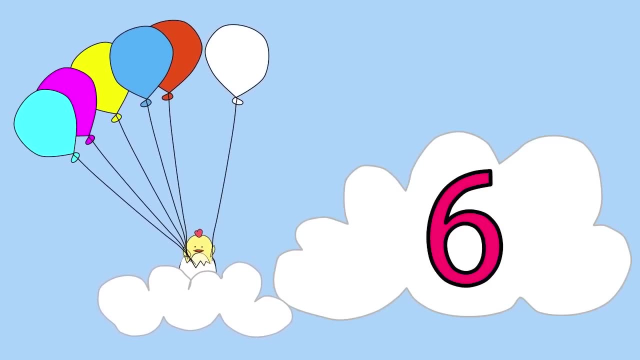 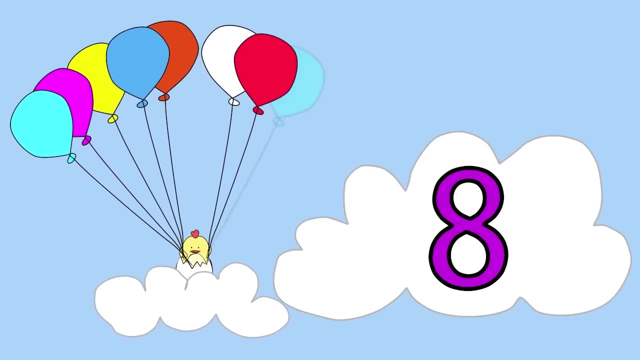 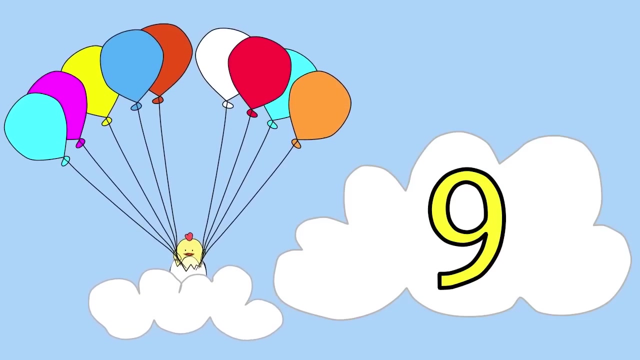 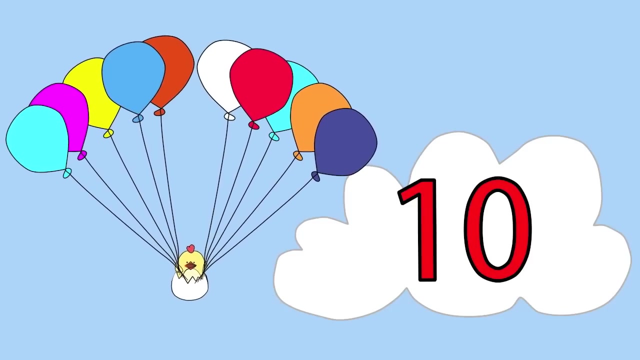 4,, 4., 5,, 5., 6,, 6., 7,, 7., 8,, 8., 9,, 9., 10,, 10. Great, Now let's count from 10 to 1.. 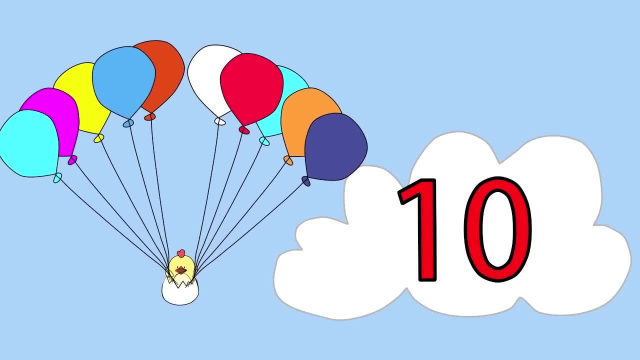 10,, 10. 9,, 9. 8,, 8., 7,, 7., 8,, 8., 9,, 9. 8,, 8., 7,, 7., 8,, 7..